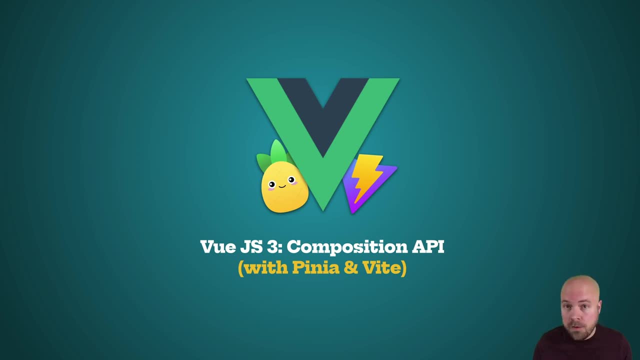 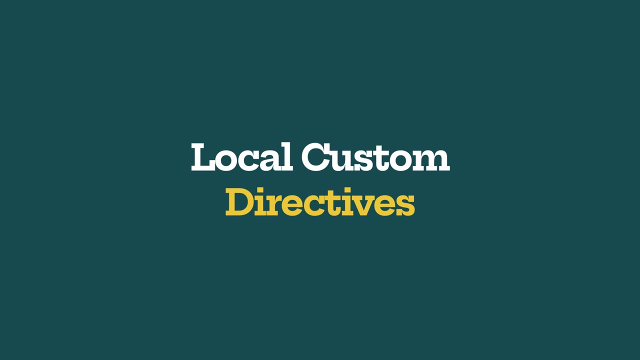 an individual component and global directives that can be used anywhere. in our app. You can find a link to the whole playlist down in the description and you can grab the full course with my discount at dannyslink. composition API Vuejs is full of directives out of the box. 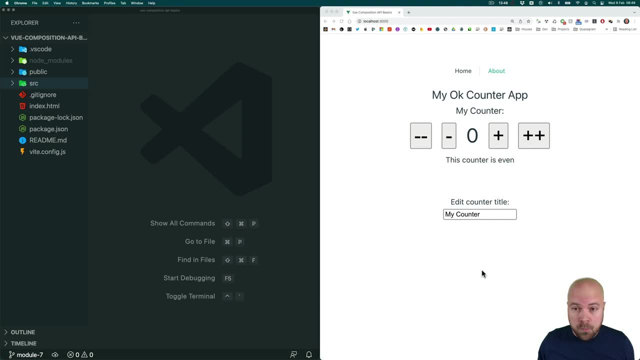 such as vmodel, vshow, vif, etc. But we can create our own custom directives to add functionality to elements, so that we can do something to an element once it's been created or mounted. A classic example is to create a directive which autofocuses. 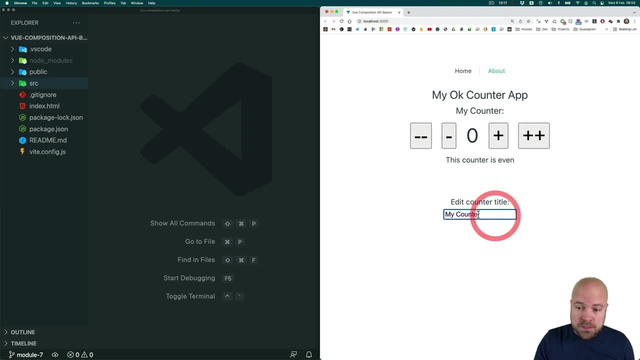 an element. If you want to create a directive that auto-focuses an element, you can create a directive that auto-focuses an element. If you want to create a directive that auto-focuses an input field, So let's create a directive which auto-focuses this input. on our home view. 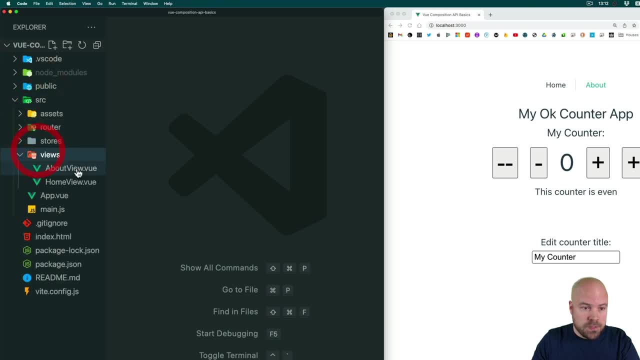 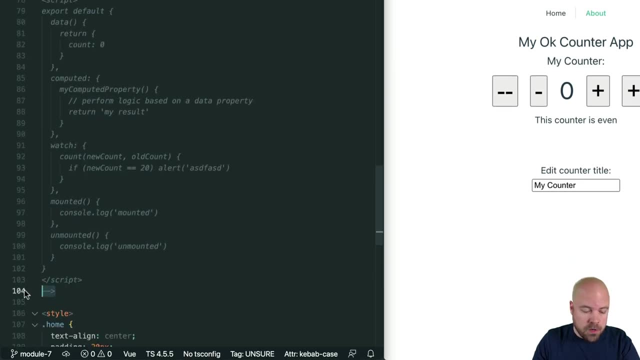 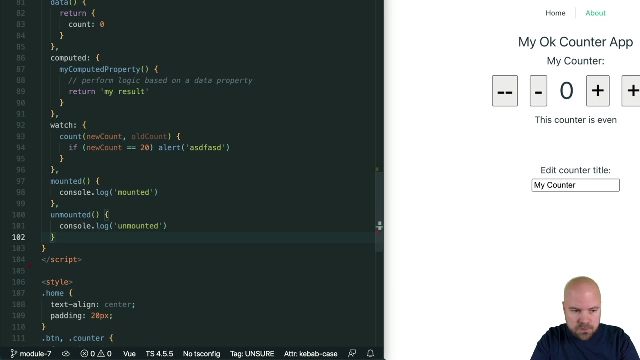 So I'm going to jump to the home view in source views and home view dot view. and let's remind ourselves how we do this: the options API way. So I'm going to uncomment the options API code and in the options API we had to add a directives. 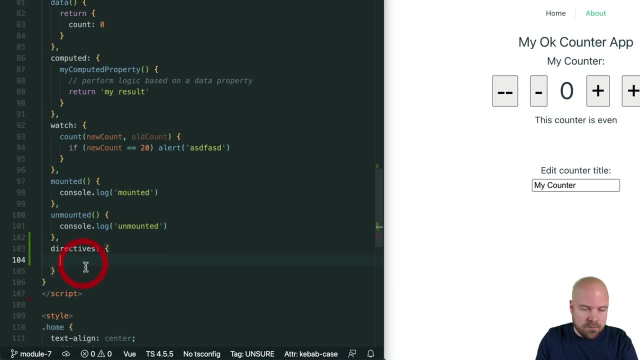 option which is an object, and we could place all of our directives in here. So let's create an autofocus directive, so we could call this autofocus and again we set this to an object and inside here we can add any hooks we want, such as created or mounted. So let's add a. 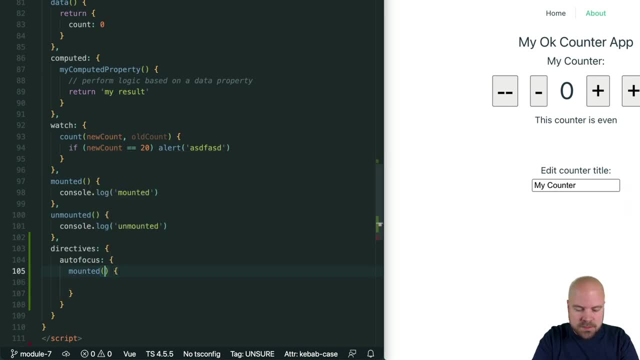 mounted hook and we can get access to the element by passing in this l parameter and then we can do something with that element and in this case we want to focus it. so we can do lfocus and I'll save that and we should now be able to use that element. So let's create an auto focus directive. 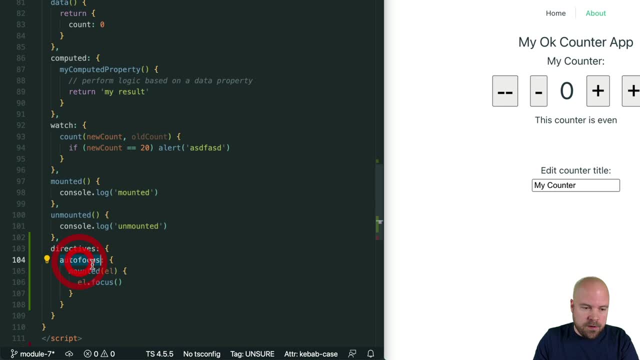 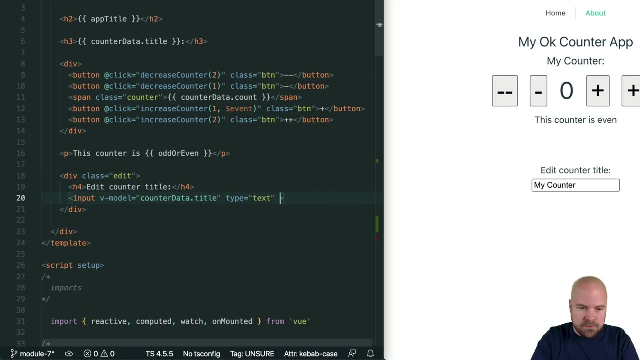 So let's use this directive on our input and we just need to prepend whatever name we've used here with v dash. so if I jump up to the input which is here, we should be able to just add v dash, auto focus, and this should still work even though we're using options API here. so if I reload the page now, 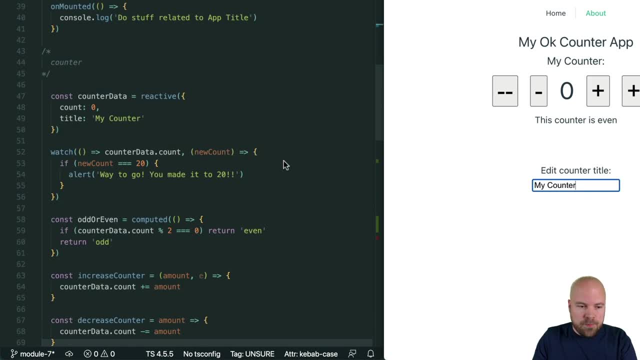 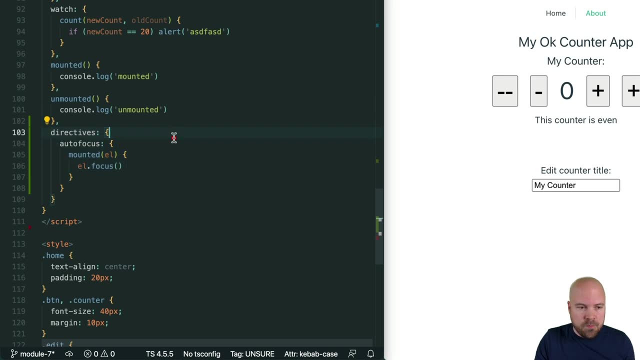 you can see, it's auto focused, this input. so, with the options API, all of our local directives had to be placed within this directives object which, again, as I keep saying, with the options API, this often leads to related code being scattered across many lines of code, whereas 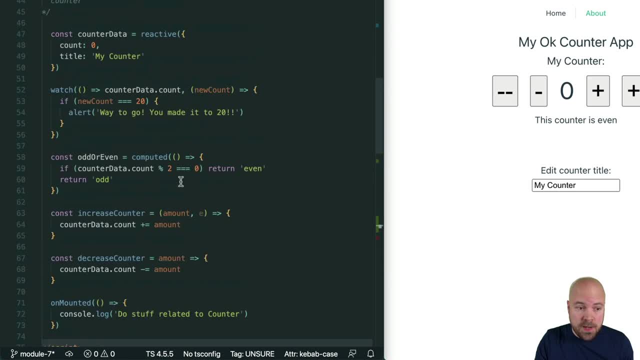 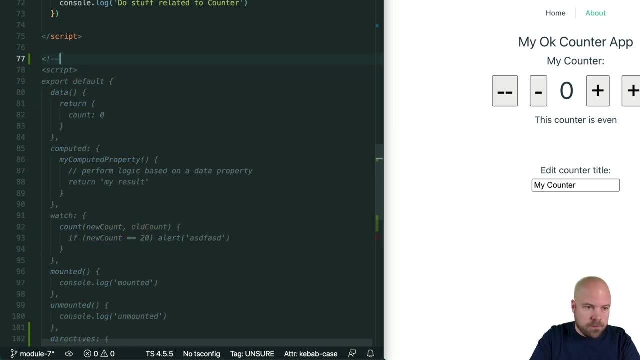 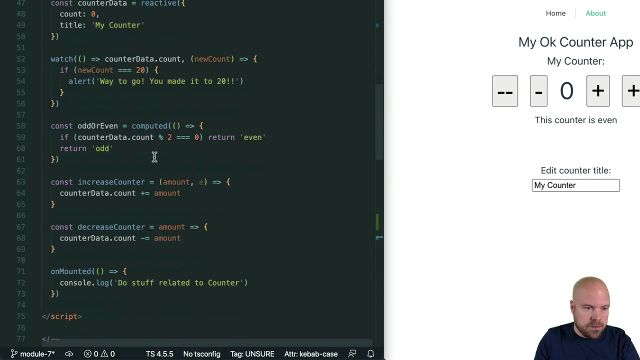 with the composition API we can create a local directive anywhere within our setup function. So let's comment out our options API code and do this the composition API way. So I'll just comment out this script section and jump up to our composition API script section. 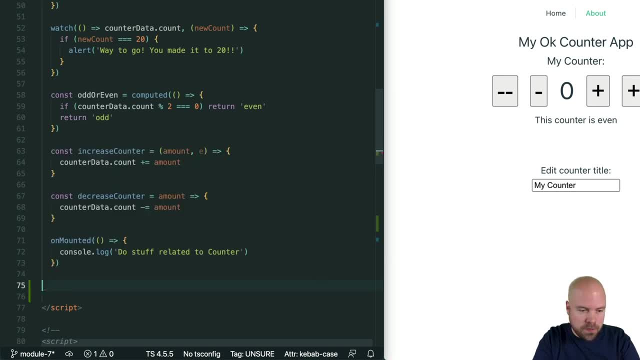 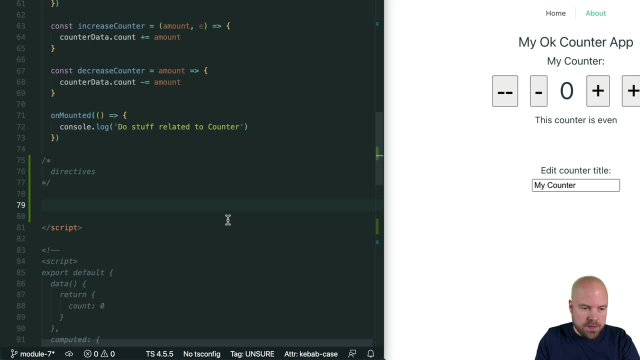 and at the bottom I'm going to add another one of these block comments called directives. and to create a directive we need to create a const and the name of this const needs to be camel case and it needs to start with a lowercase v, so we might call this v auto focus and whatever. 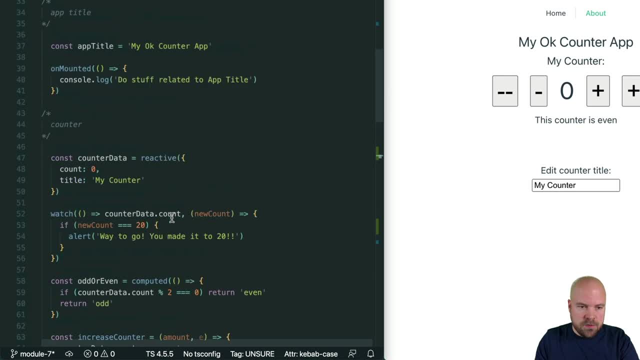 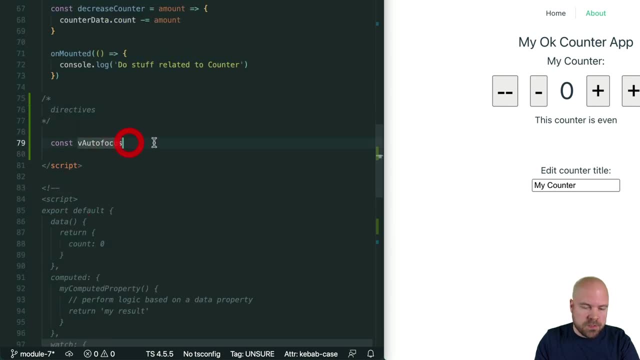 name we use here will determine the attribute that we actually use, although it will be converted into dash case like this. so v auto focus- camel case becomes v dash- auto focus if we want to set this to an object, and inside here we can add a life cycle hook, such as created: 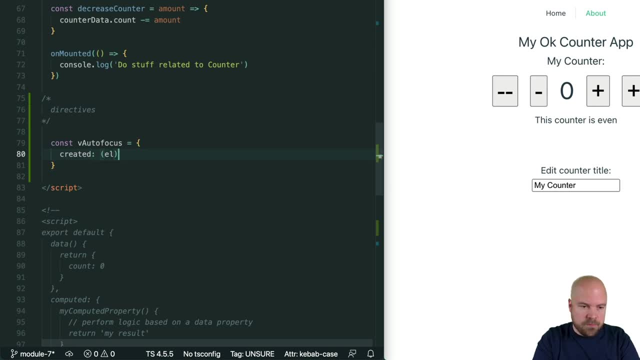 and we set this as a property which is set to a method like this, and we can then do something with the element which we've added this directive to in this created hook, and we can also use all the other hooks as well, such as before mount and mounted and before update. So this is the first step for this project. We're going to go ahead and click on this one. We're going to go ahead and click on this one And we're going to click on this one, And we're going to click on this one. 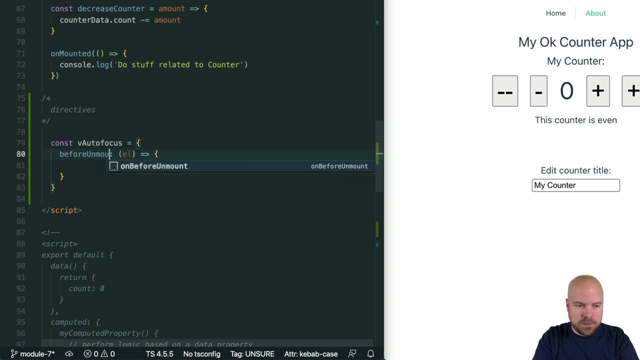 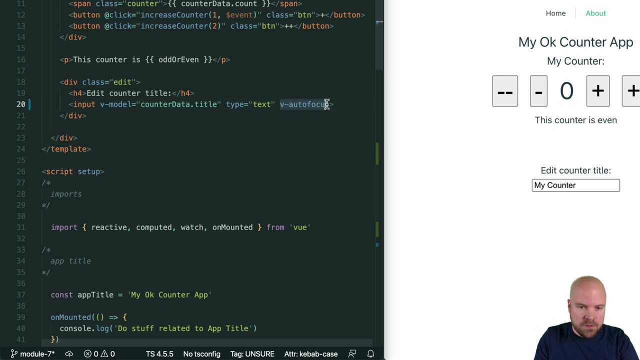 And we're going to click on this one and updated before unmount and unmounted. but for this let's use the mounted hook and again, we can just use the same code we did before to focus this input: l dot focus, and we've already added this directive to this input, so this should hopefully be working now. 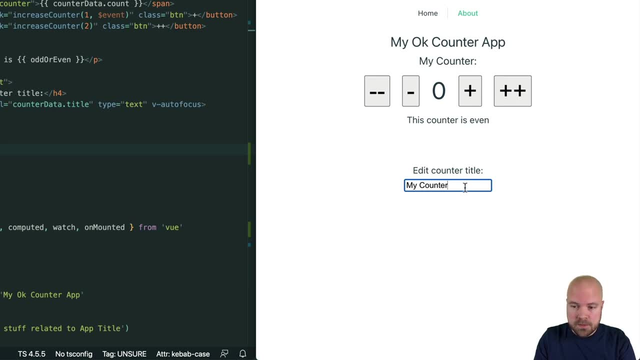 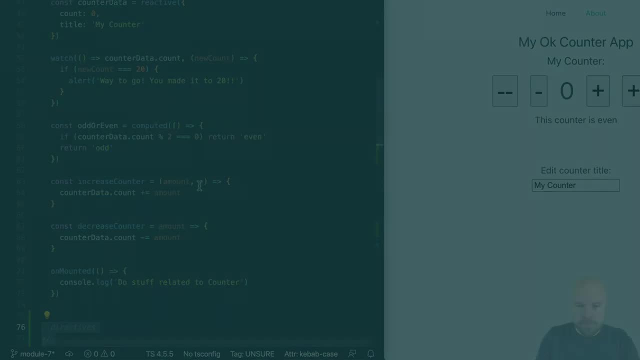 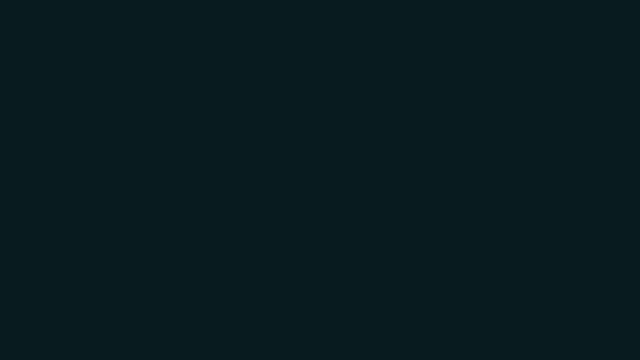 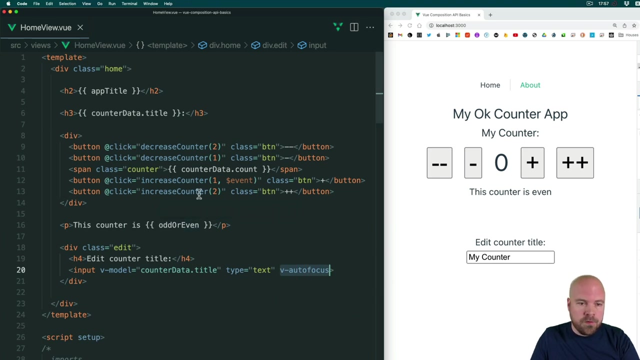 i'll just reload the page and, yeah, it's still auto focusing this input, but now we have the freedom to place this local directive anywhere we want within our script section. right now we can only use this- the auto focus directive- on this particular component- home view, dot view- if we want to be able to use this directive throughout our app on different. 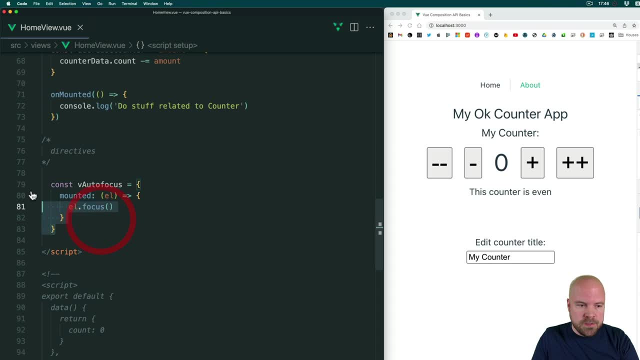 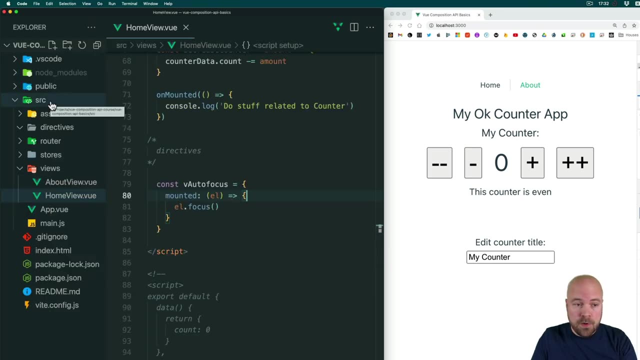 components. then we can take our directive and put it into its own file and create a global custom directive. so let's jump to the file explorer and we'll create a folder where we can place our custom directive. so i'm going to create a new folder inside the source folder called directives. 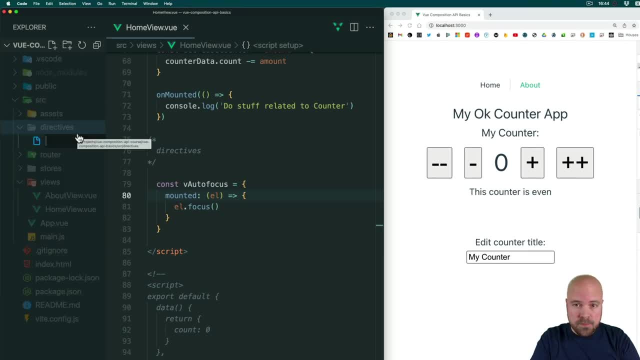 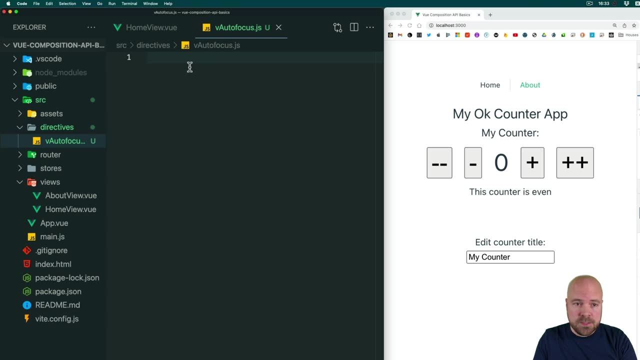 and i'm going to create a new file and let's give this file the same name as our directive. so v autofocus dot js. and, by the way, if you have issues with your tab spacing here, because all of these files in this project that we created have a tab space of two spaces, you might find that when 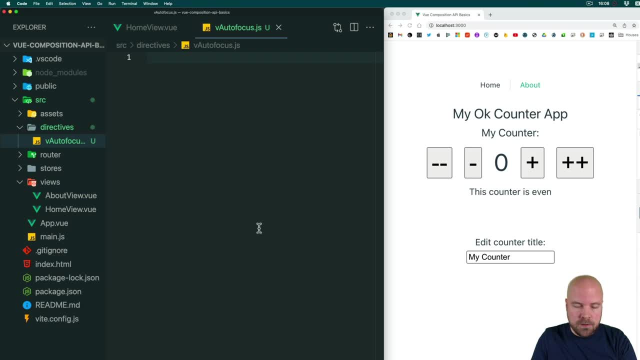 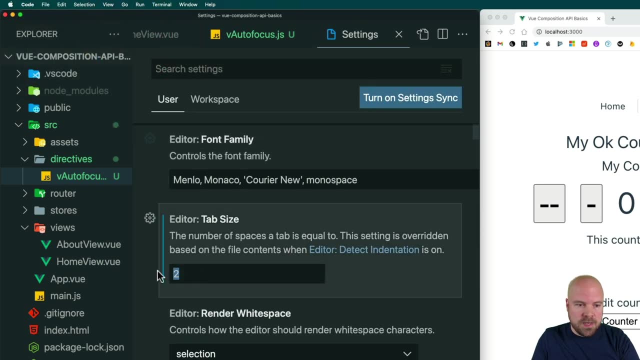 you create a new file, it's set to four spaces because that's the default in vs code. if you want that, just go to code and preferences and settings and just change this tab size setting to two and you may need to just delete this file and recreate it as well, this v autofocus file. but anyway, let's. 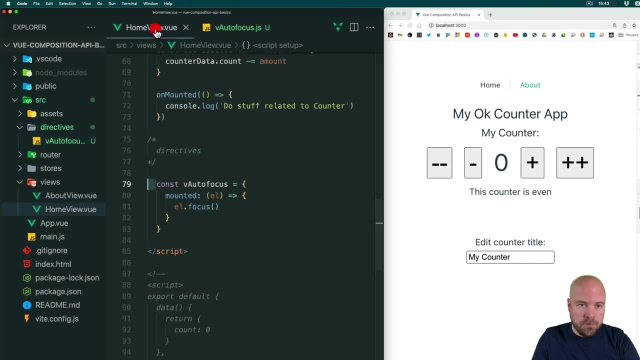 move our directive into this file. so i'll jump back to homeviewview. now we can just cut this code and i'll delete the comment as well, and we can jump to the autofocus js and just paste that in, and all we need to do to make this available to other files is export to the v autofocus file. 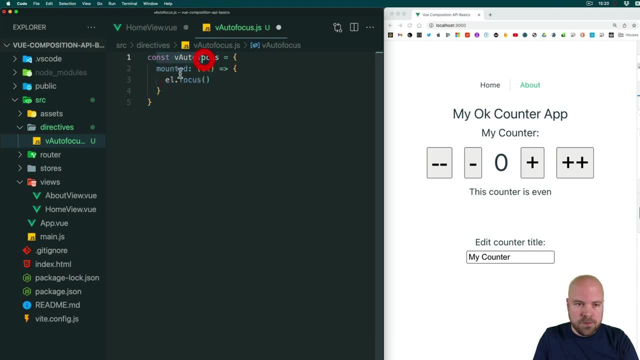 and we can just paste that in, and all we need to do to make this available to other files is import this const. so we can just add export at the start and save that. and now, if we jump back to homeviewview, we can now import this directive and use it. so i'll just jump up to the import. 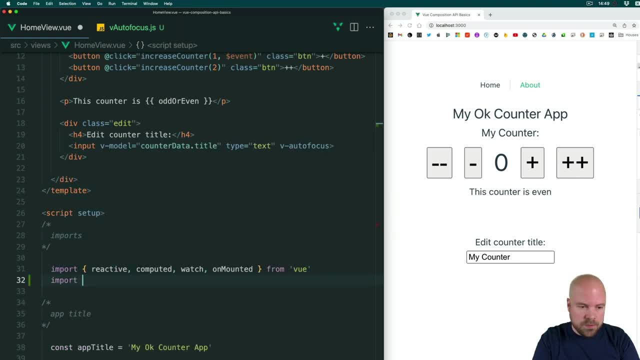 section and to import this directive, we can just do import v autofocus from at slash directives, slash v autofocus, and we already have our directive added to this input. so this should hopefully be working. i'll reload the page. and yeah, it's still working, except this is now a global directive that we can use anywhere, so 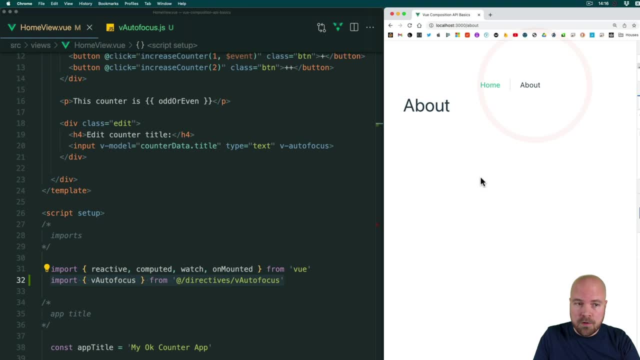 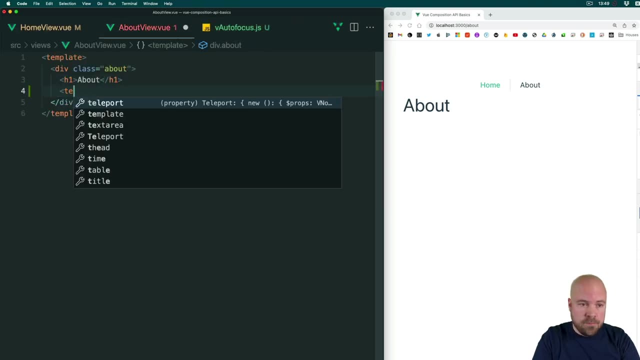 just to demonstrate that, let's add a text area to our about page. so let's open up the about page- source views, about viewview- and we'll add a text area after this heading and then we need to add our script setup section and i'll add a comment for.